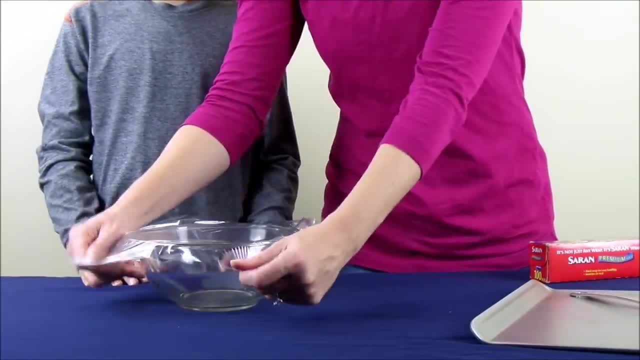 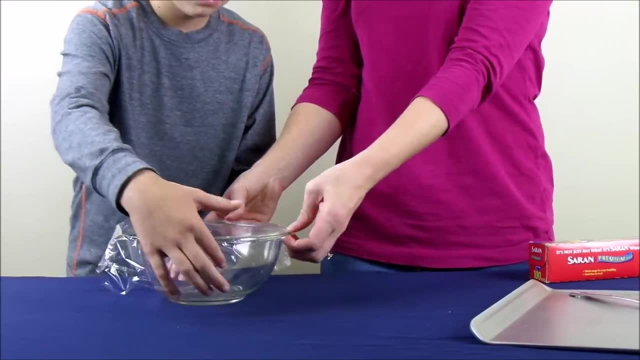 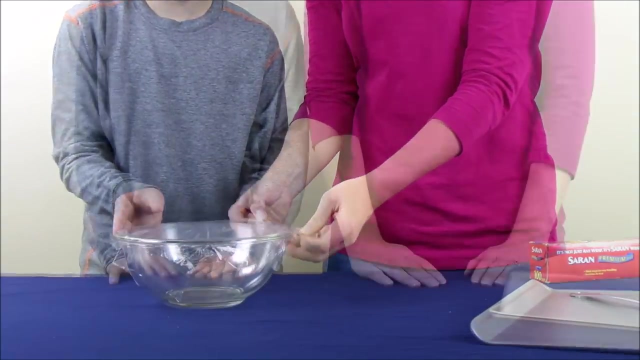 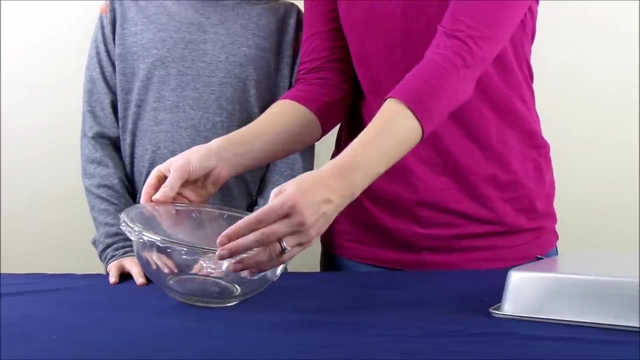 it on top of the bowl. You're going to make sure the saran wrap is very tight on the bowl. The most important thing with the saran wrap is that you get it very tight across the top of the bowl, so take your time when you're positioning it. Once you have it tight, you're ready to move. 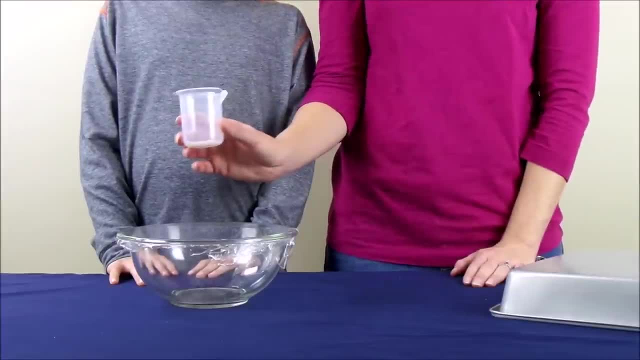 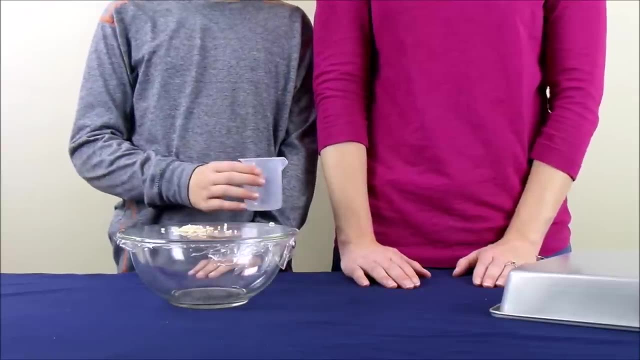 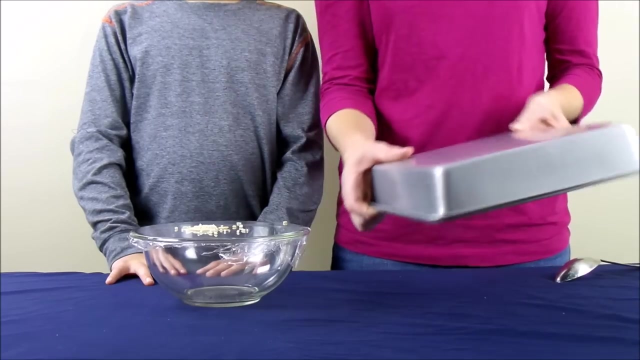 on to the next step. This is where you're going to take some uncooked rice and you're going to pour about a teaspoonful on the top of the saran wrap. Once the rice is on the saran wrap, you're going to take a metal tin. You can use a cookie sheet or in my case it's an 8x11 pan. 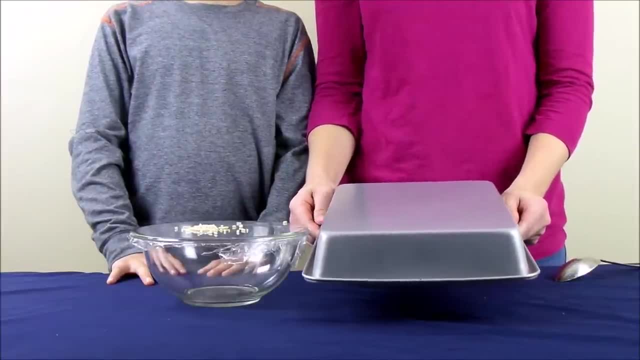 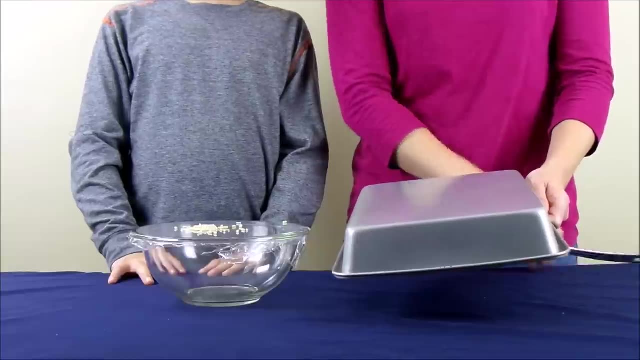 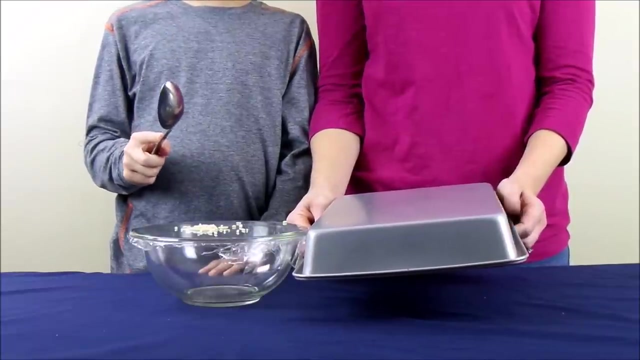 and you're going to position it close to the bowl. The important thing is that you're holding it in the air and then again, that it's very close to the bowl itself. Now I'm going to give my son a metal spoon, and what he's going to do is he's going to hit the metal plate, metal tin, and we 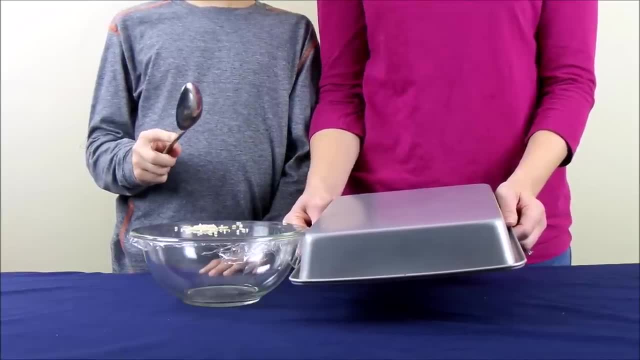 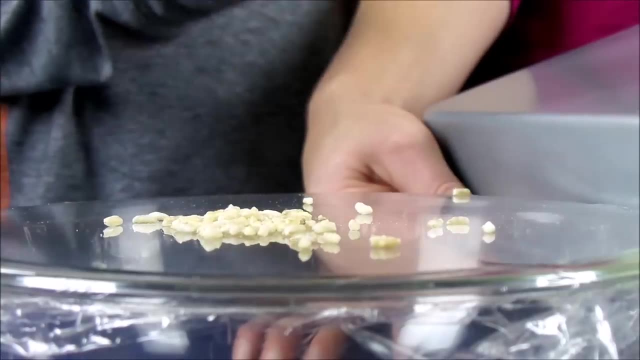 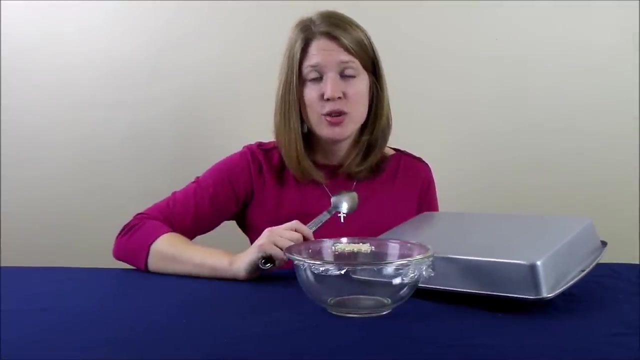 are going to hear the sound and we're also going to see some sound. You're going to hear the sound and you're going to hear the metal dip, and you're also going to hear the metal snap and saw something happen. Can you tell me why, when I bang on the metal pan, the rice moves? 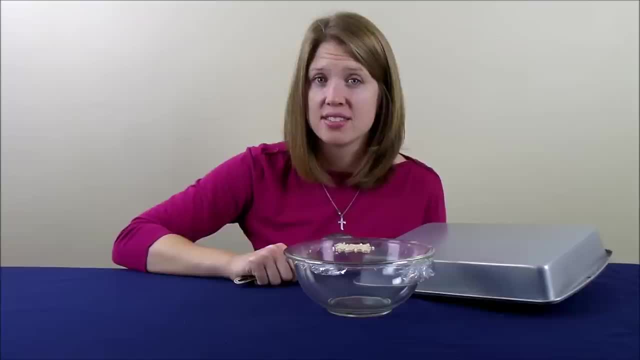 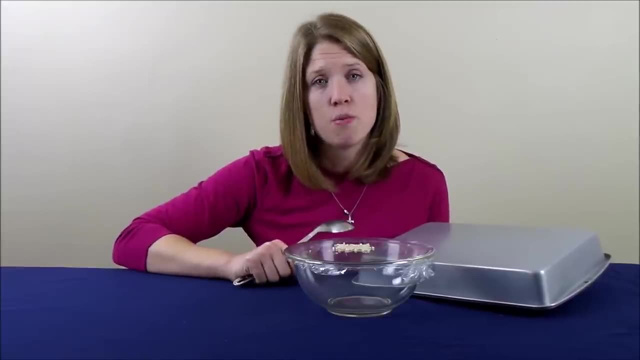 Leave a comment below to submit your guess and visit Cool Science Experiments headquarters dot com to find out the answer. You'll be able to print out instructions for this experiment and you'll find videos of more science sleight of hand information on my blog. at Cool Science Experiments Headquarters dot comazuje. you'll be able to print out instructions for this experiment and you'll find videos of more science sleight of hand information on my blog, ScienceS중에com. and if you go online to find something drinkable when you do this Easy. 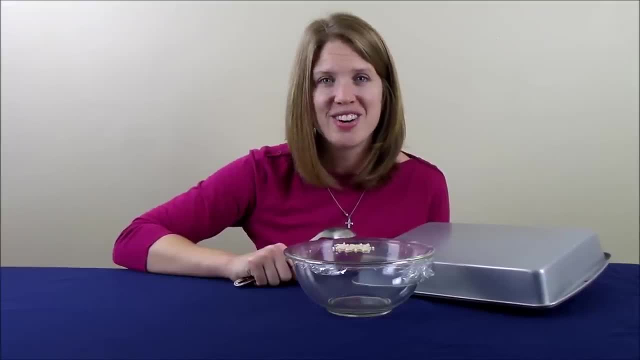 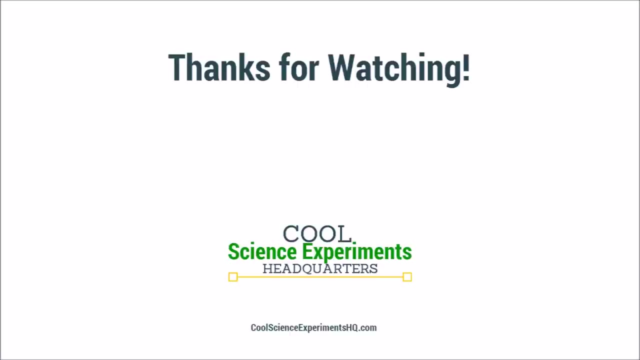 experiments that you can do at home too. Thanks for watching everyone, and we will see you next time. We hope you enjoyed the experiment. Click the button to sign up for our free email. Then we will send you a fun new experiment each week. See you next time.